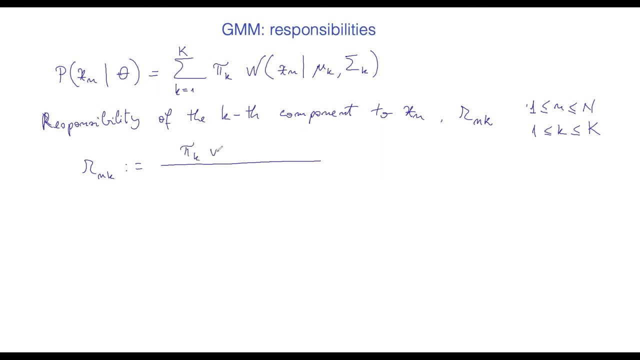 It's going to be IK times the normal distribution with mean mu K and covariance matrix, sigma K, over the whole, So that this is normalized over the whole thing. So this is from sum 1 to K by J and normal distribution of Xn, given mu J and sigma J. 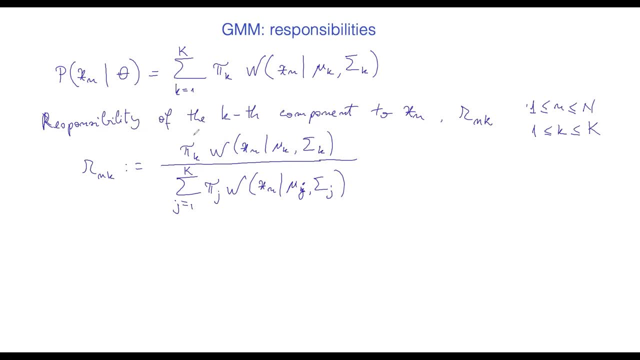 And obviously this is going to be proportional to this part, to the likelihood of this one, And also obviously this is going to lead to a matrix. So we are really collecting these responsibility. So maybe I'm just writing here the responsibility matrix is going to be made of all. 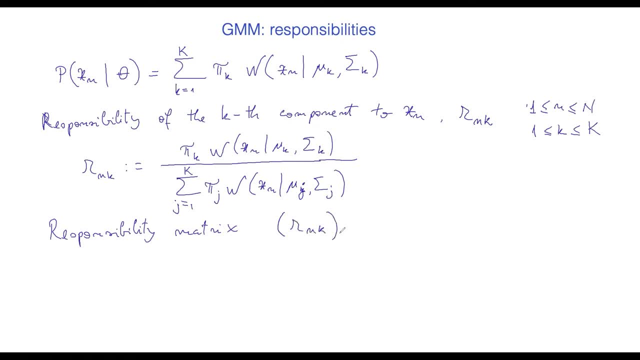 these responsibilities. So it's going to have N rows and K columns And if I take the, the sum over one row, So sum over a row is always one, And that's because we are normalizing this thing. And so when we take the contribution of all the components to a data point, 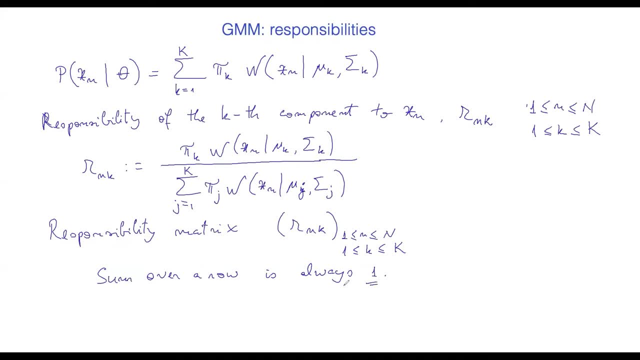 and normalize, this is always going to be 1.. So, in other words, sum of R and K, sum over K, is always going to be 1.. And also, obviously, these numbers. they are all greater than or equal to 0.. 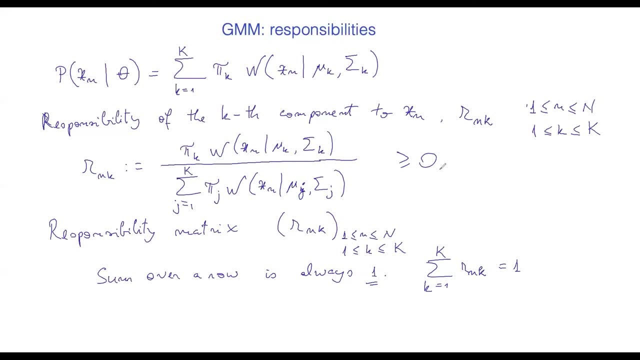 Now the way you can think about it, just realizing that they sum up to 1, you can think about this Rn. So this leads to the idea of Rn as a sort of a soft assignment Of Xn to the K mixture components. 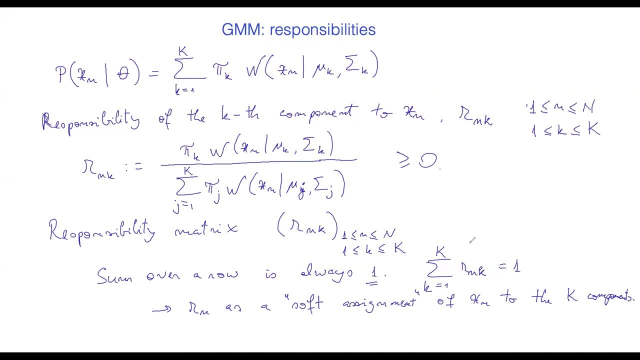 So what I'm saying here is that, realizing that they sum up to 1, you can think about it as, by the way, this Rn is just the collection of all these points in here. So if I'm just, I'm collecting these Rn1,, Rn2, and so on, Rn- capital K. 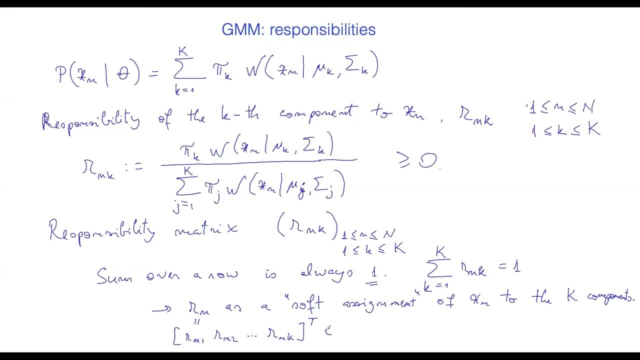 And I take this as a vector column, as usual. So the way you can think about this is really a soft assignment kind of thinking. what's the likelihood of that point belonging to each one of the clusters if you have to think in terms of clusters? 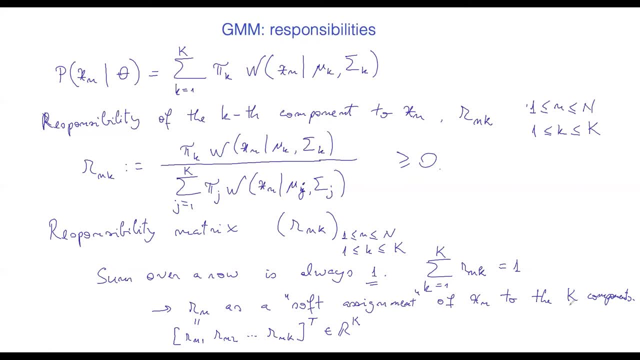 So soft assignment of these data. So the Rn1, Rn2 log-out point to these components And it's going to be given the weight of that assignment. it's going to be given by each one of these components: Rn1, Rn2, and so on. Rn k. 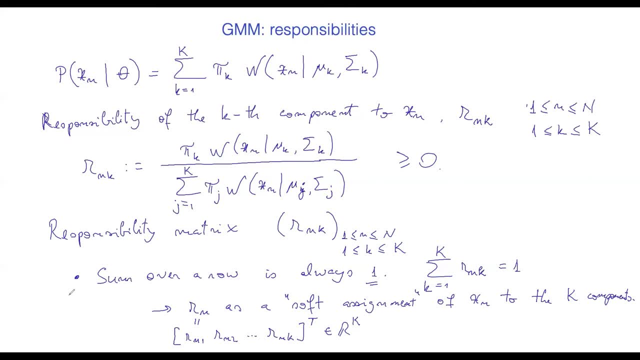 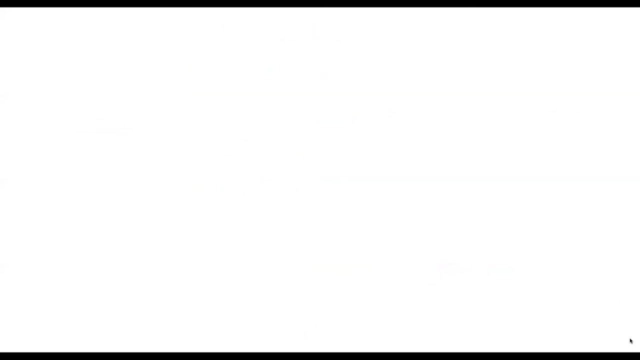 For the sum. sum over a row is always 1.. And we can also think about the sum over a column, which is going to be component to the overall data set that you have. I want to give you just this matrix of responsibilities. 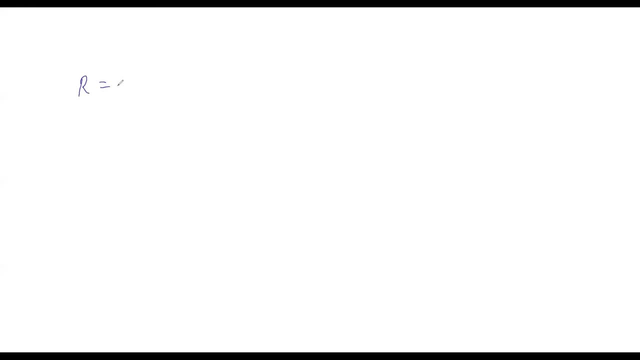 So the responsibility matrix for that running example we have in this chapter- and you can check it in the very first video we had in this series of lectures on Gaussian model, mixture models, And that's going to be a matrix that has obviously three columns. 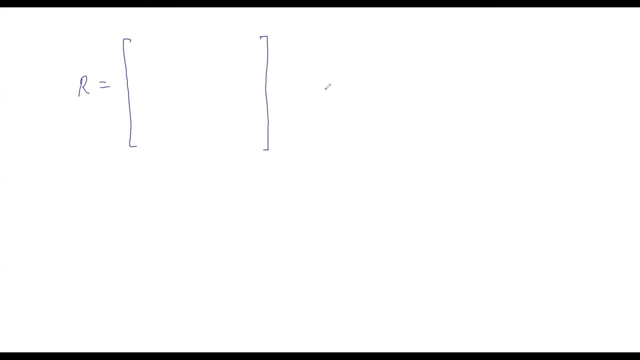 because we have in our running example three components And we had in that example we had seven data points. So this is going to be a matrix, seven by three. And when we calculate this matrix, these values we are going to get. this is one zero, zero. 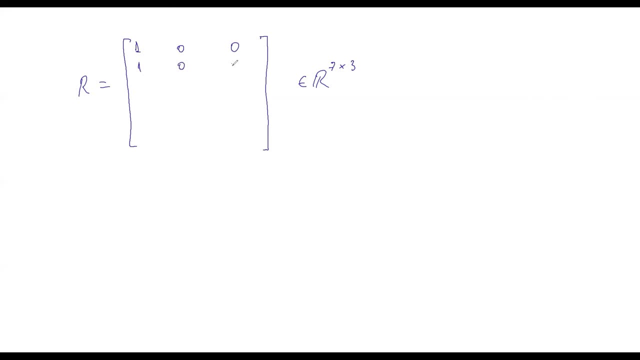 And we have one zero, zero, zero, zero, fifty-seven, zero, nine, four, three and zero, Zero, dot, zero, zero, one, zero, dot, nine, nine, nine and zero. here, These ones are all zero.